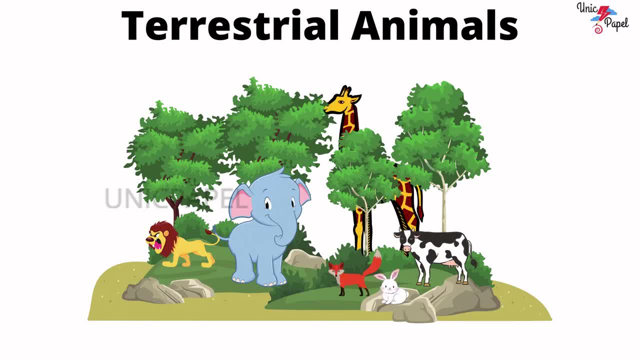 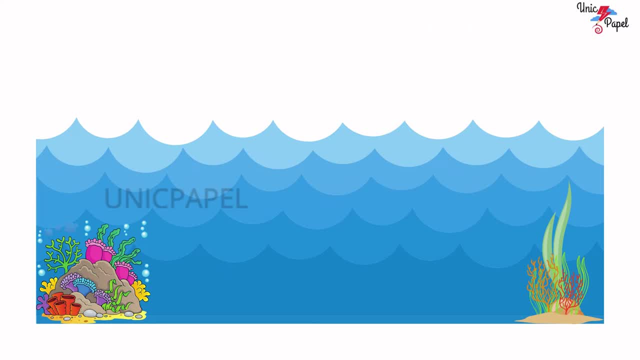 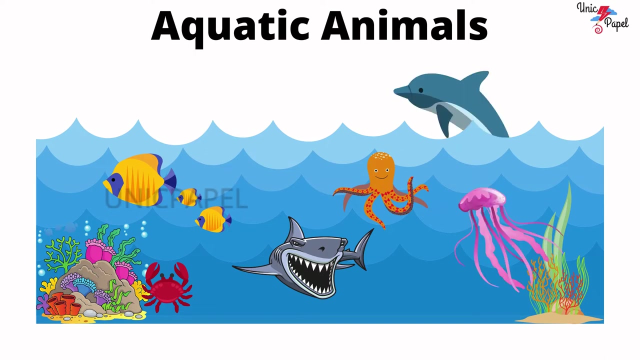 Giraffe, Rabbit, Dog and many more. Next, Aquatic Animals: The animals that live in water are called Aquatic Animals. Example Fish, Crab, Octopus, Shark, Jellyfish, Dolphin and many more. Next Aerial Animals. 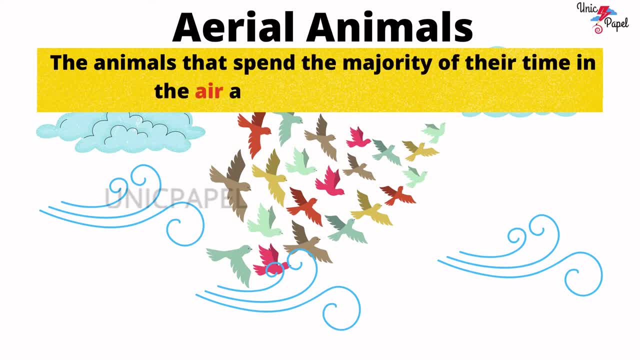 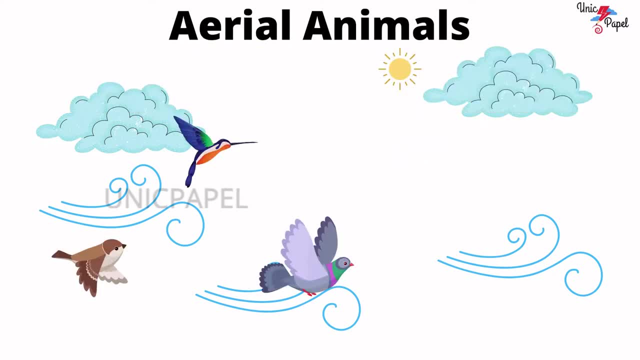 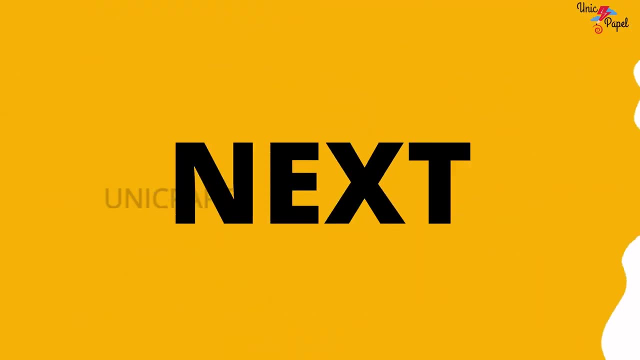 The animals that spend the majority of their time in the air are called Aerial Animals. Example: Sparrow, Kingfisher, Pigeon Crow, Eagle Bat and many more. Next Arboreal Animals: The animals that spend the majority of. 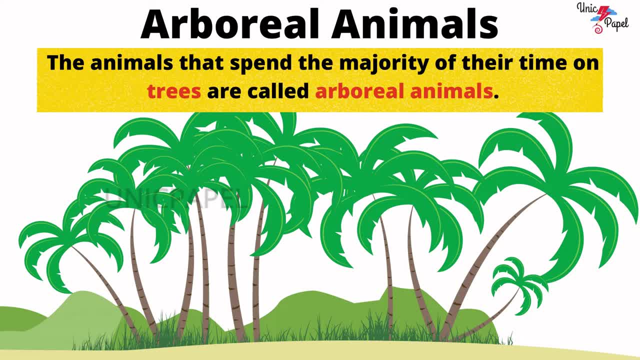 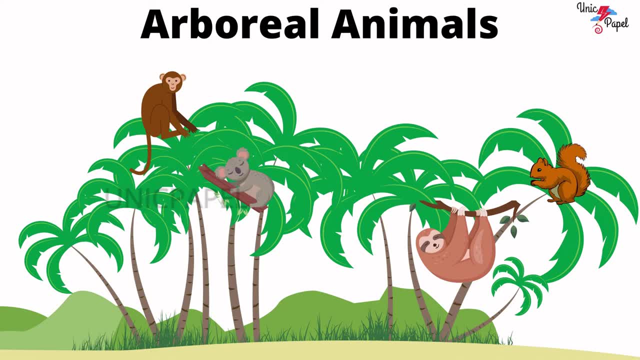 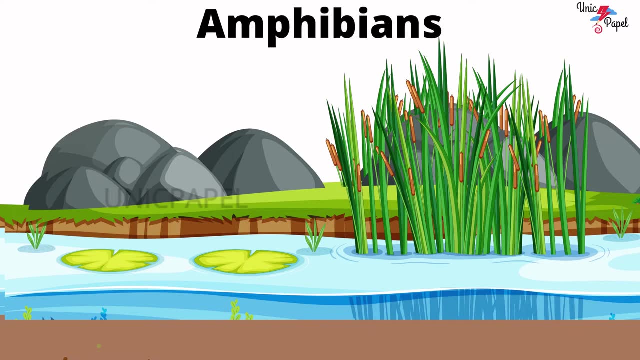 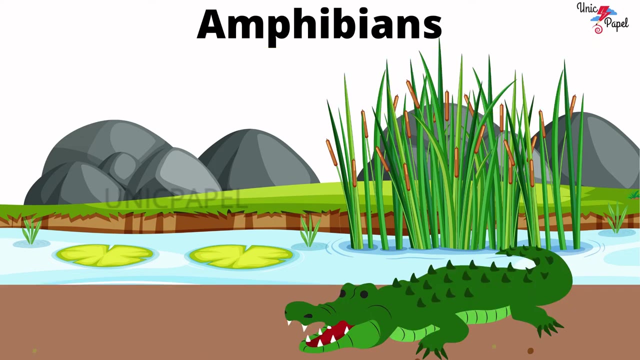 their time on trees are called Arboreal Animals. Example: Monkey, Squirrel, Sloth, Koala, Tree Snake and many more. Next, Amphibians: Animals that live both on land and in water are called Amphibians. Example: Daniel, Crocodile, Frog, Snake. 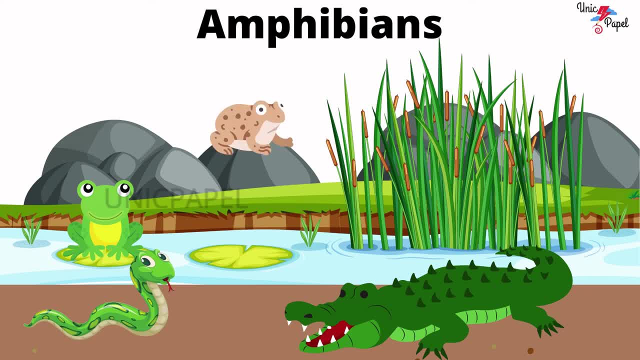 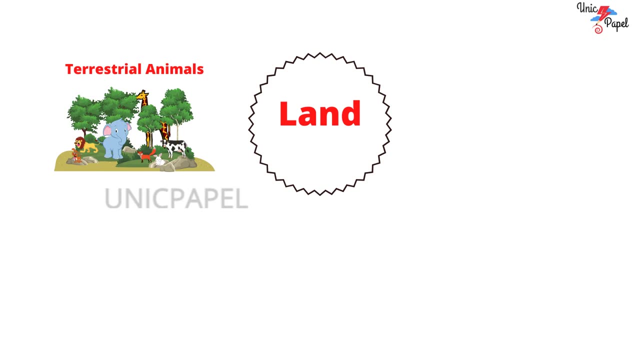 Toad Newt and many more. Example: Daniel: Crocodile Frog, Snake, Toad Newt and many more. Next: Crocodile Fork, Snake, Toad Newt and many more. Next N initiatives. The animals that live on land are called: 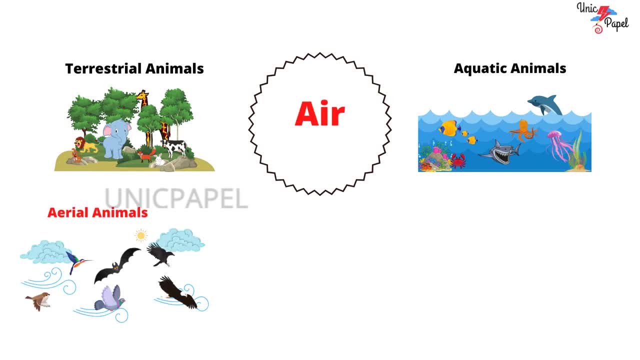 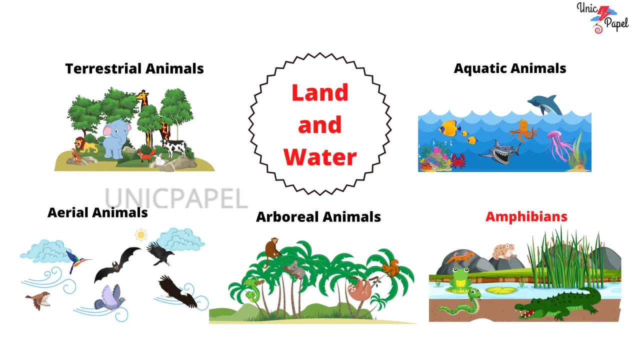 Animes. Terrestrial Animals- The animals that live in water, are called Aquatic Animals. animals, the animals that spend the majority of their time on trees, are called arboreal animals. animals that live both on land and in water are amphibians. well done, kids. keep practicing. click the upcoming video to 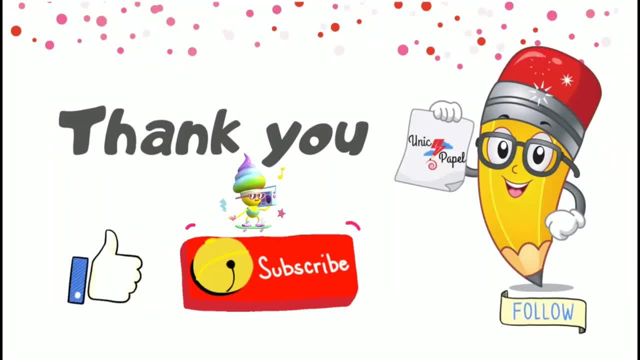 know more about animals. thank you for watching Munich paper. be sure to subscribe and like our video. you.